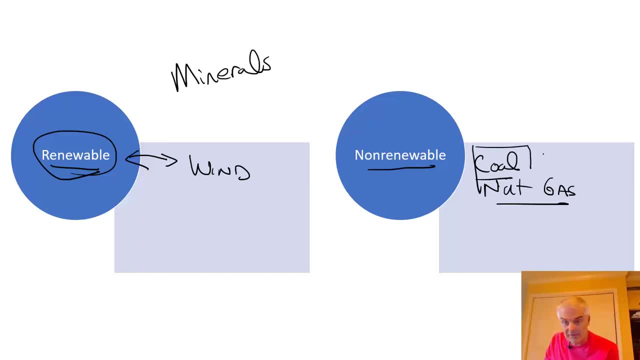 but they're not. they're going to be depleted at some point, And so there's a lot of concern about this. oil, natural gas, et cetera- and wind is not. We're really focusing here on the concept of minerals. Now, minerals inwardly, you can consider. 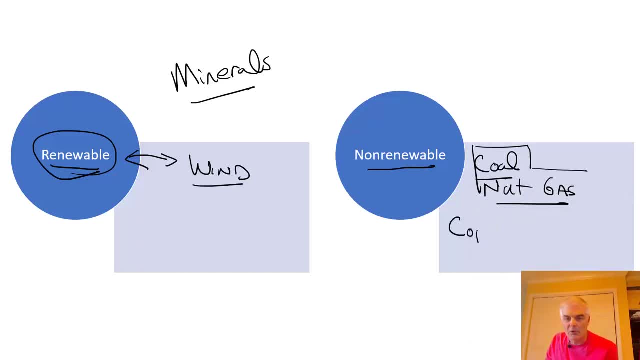 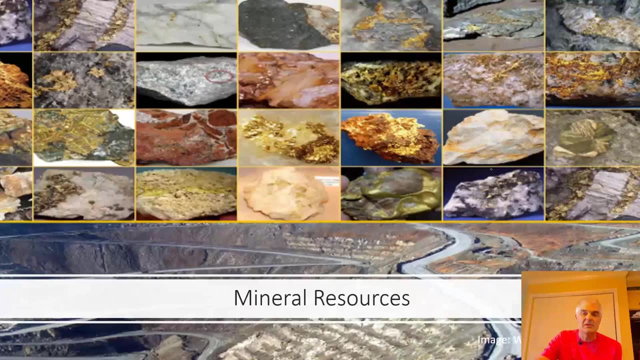 oil and natural gas as a mineral, but we're thinking about things like copper ore or something like that, because there's certainly only so much that's in the Earth And, as we're going to find out, there's actually an issue is that they're not always in the same places. So here's some. 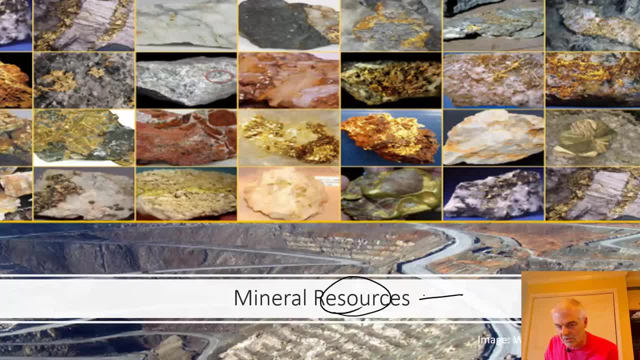 examples of mineral resources. Now, when we talk about mineral resources, we're talking about minerals that are valuable, right? So what the heck is a mineral resource? It's a. it's like going to be something you're going to find in enough concentration, and it's useful for. 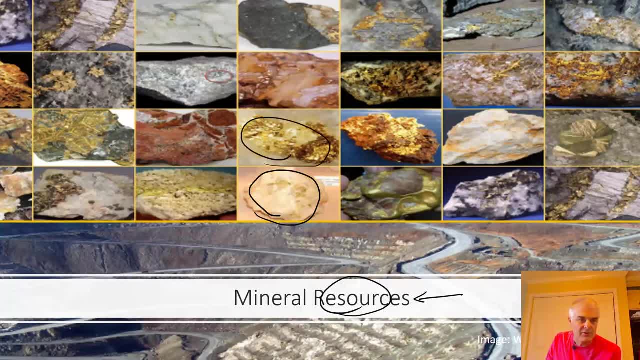 you to discover it right. So I mean classic picture of gold. These are some pictures of some different valuable minerals that are useful for the world right, And there may be other minerals that we know about that at some point will become valuable. but you have to have a reasonable. 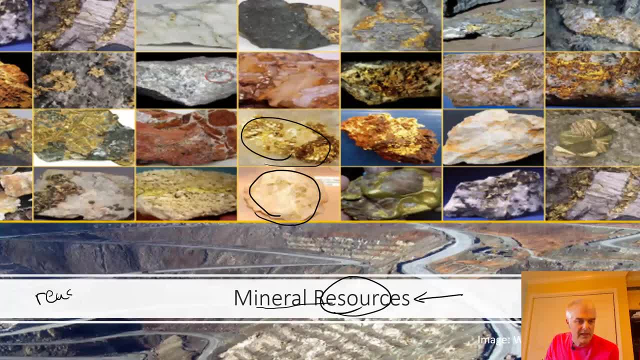 expectation- You should probably jot that down- A reasonable expectation. I'm basically making some money off of the deal, right? Because you're going to dig it up out of the ground and then you're going to have to extract it, which is going to cost you some money, And 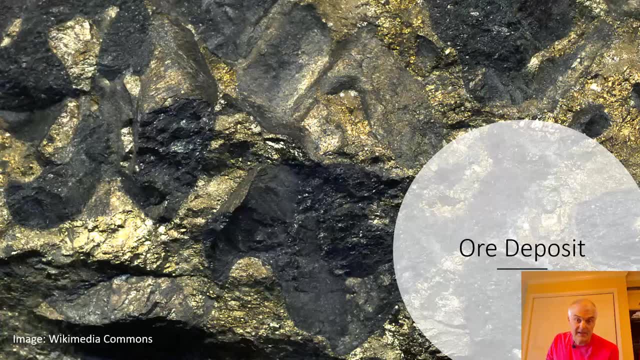 then you're going to have to then sell it, et cetera. Now you find these in things called ore deposits. An ore deposit is usually a rock. Remember we talked earlier about this. a rock contains minerals. But if I've got, if I've got a rock, if I've got a rock, if I've got a rock. 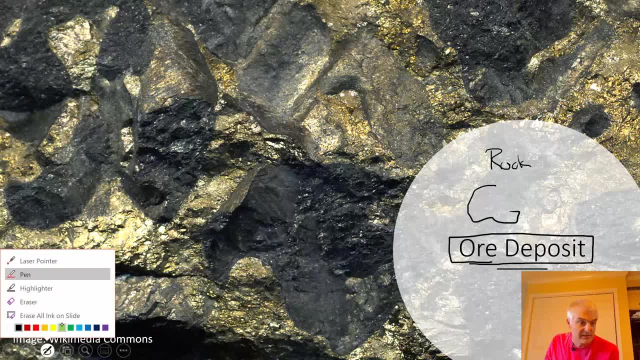 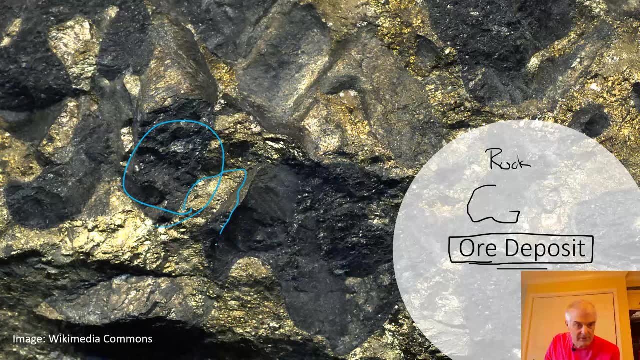 you know well, this one right here. we've got this particular image right here, And maybe the ore is actually this sort of goldy colored thing, right? So if that's the case, I'm going to have to break this up and this is just junk, this black rock here, I don't care. 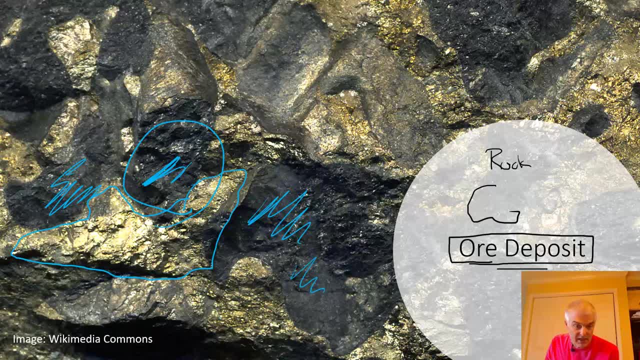 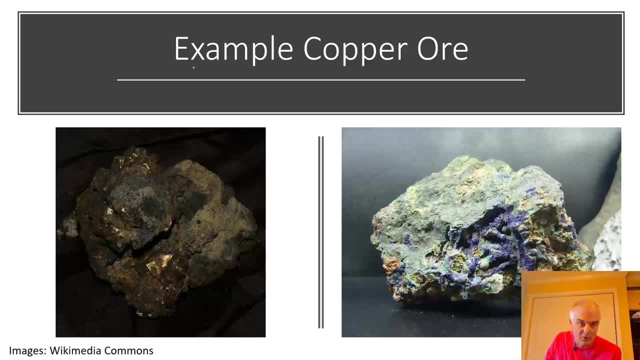 about that. Maybe it's useful for something else, but if the valuable rock is this goldy thing, then I need to find a way to extract it. So let's take the example of copper ore. All right, Here are two different ore containing rocks that both have copper in them. Notice they? 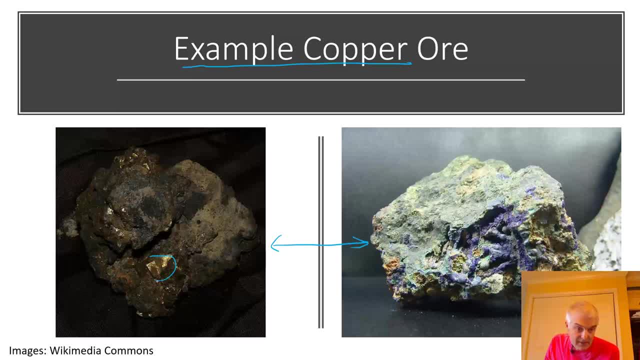 look very different. The one on the left. here's the copper ore that matters. You can kind of see little specks here, And on the right it's actually it's the bluish stuff. So it's a different ore And so the chemistry, if you will, of this ore body and how you get that copper out. 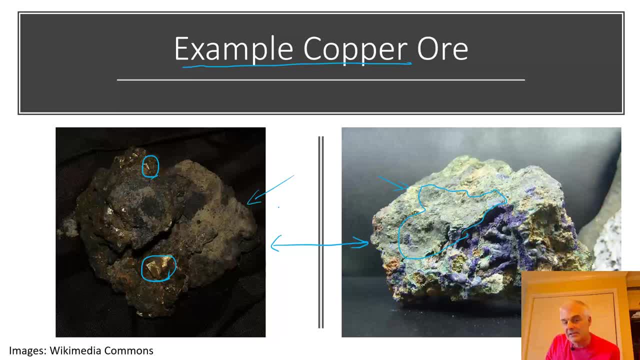 of this one compared to this one is going to be significantly different. But so other things about copper: interesting: It's 0.01.. 0.01% of the earth's crust, But as of right now- 2019, they're saying that you need about 2.35%. 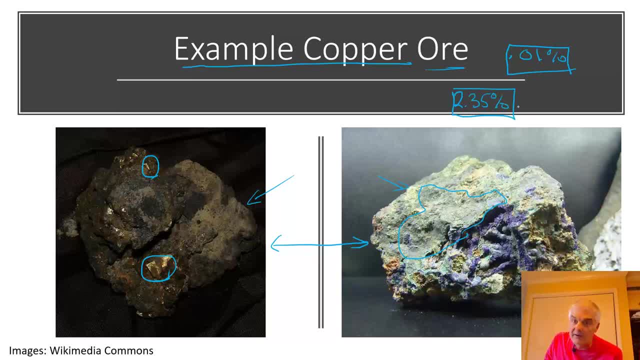 minimum of a rock or of a ore for it to be economically feasible. Does that make sense? So this is average in the earth. So that leads the geologist to go on a mission to explore the world to find places where the amount of copper in a body of ore is greater. 0.01% of the earth's crust, But as of right now, 2019, they're saying that you need about 2.35% of the earth's crust. But as of right now, 2019, they're saying that you need about 2.35%. of the earth's crust. But as of right now, 2019, they're saying that you need about 2.35%, And that's the tricky thing. you're trying to find out. And so, Monzo, say, when did it? 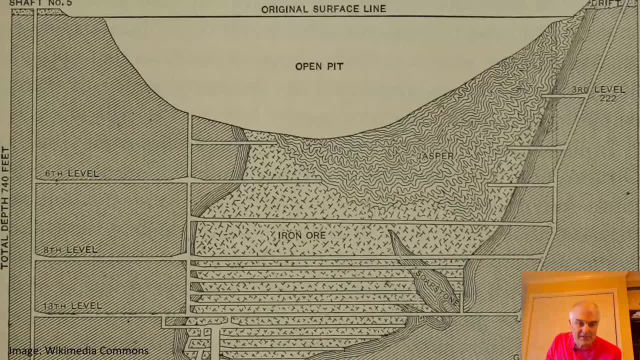 And so they study it and they look at things like maps like this. 1 thing that a scientist is, And so they study it and they look at things like maps like this. So one thing that a scientist is, or a geologist in particular, is trying to do, is to map out the world. and let's say: 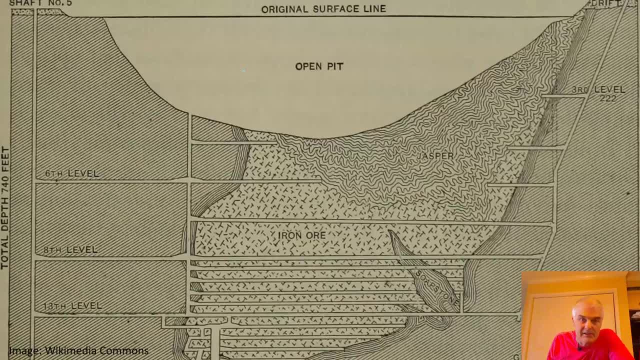 underground world, And so they've mapped out a particular area. this is a particular mine, a rock mine, And the iron is this. you see the iron ore here in this particular picture. that is where the iron is, and probably what happened is that the iron ore in the particular iron is. 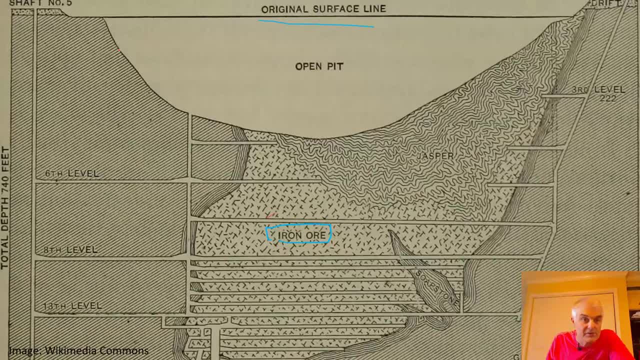 and probably what happened is in the past. you know, this is a surface pit up here there was a lot more of the iron, maybe it extruded like this and they just dug it all up, but then it narrowed down and they said: how are we going to get at that? now, this stuff over here, not important this. 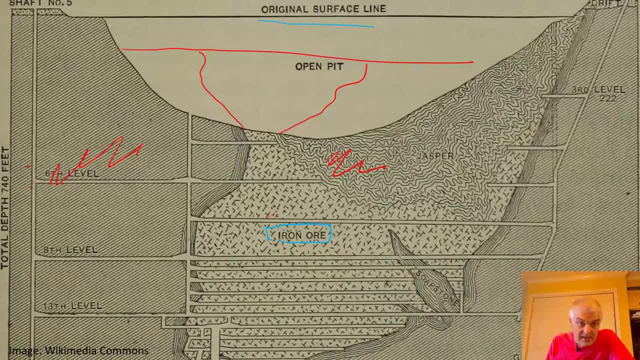 stuff over here, not important. this is where the money is, and so in this case, they've decided because when they mapped it out- and there's- we'll learn later about how they get mapped out- it's pretty cool, by the way they map it out- it gets kind of wider down here, and so what they did is: 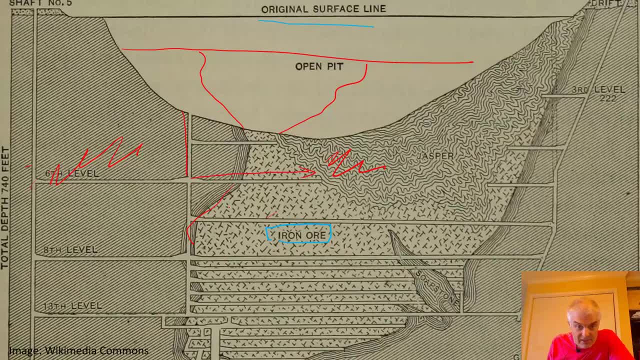 they drilled a mine. you see the mine and then they drill shafts and they start getting. you can see like the biggest best spot right here. from a depth perspective, this is where the money is right. soapstone not so valuable. so you're going to run into some impurities and you want to get places. 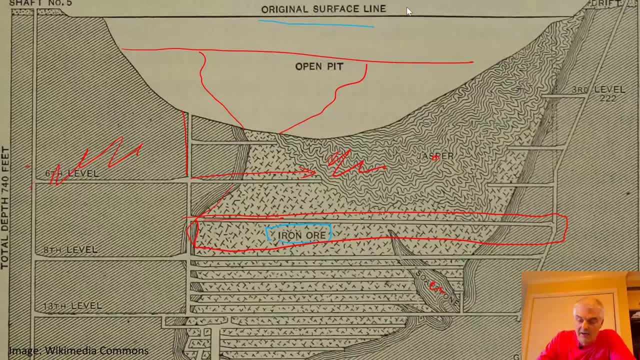 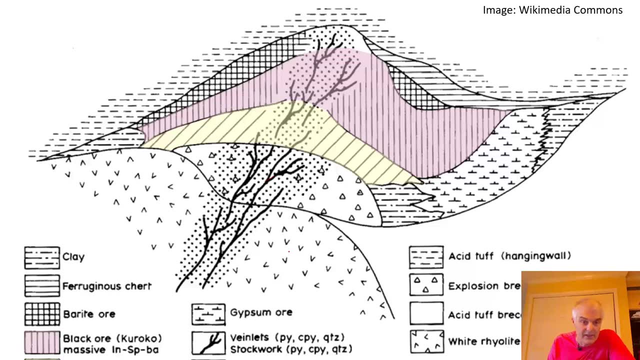 on the earth that are concentrations of the particular rocks or ores, pardon me, that you're looking for. here's another example of a different kind of one. this is gypsum ore. so that they so another underground sort of diagram of an area we're trying to find. this is the gypsum ore here. this is where the money is right, that's. 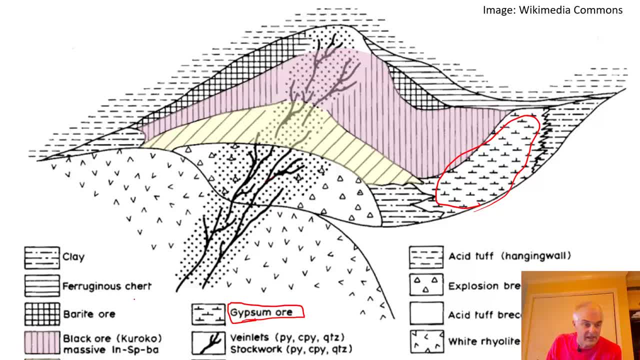 where you want to dig and so all this other stuff isn't important. all right, maybe there's maybe the barite, or how are you going to get that? so when the geologist goes in here, maybe you can get a surface mine and dig down here, but then you get about to here and then you can't. you can't just. 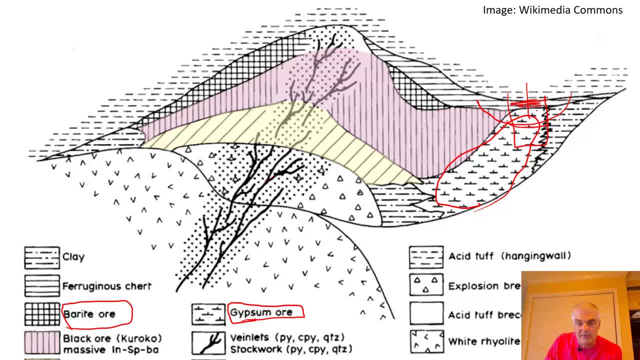 keep digging a deep hole like that. that's not possible. and at some point maybe this is going to be a good idea, but it's not going to be a good idea and then you can't. you can't just keep digging underground mine. if you're trying to get it- the barite, different kind of an ore, etc- you have to. 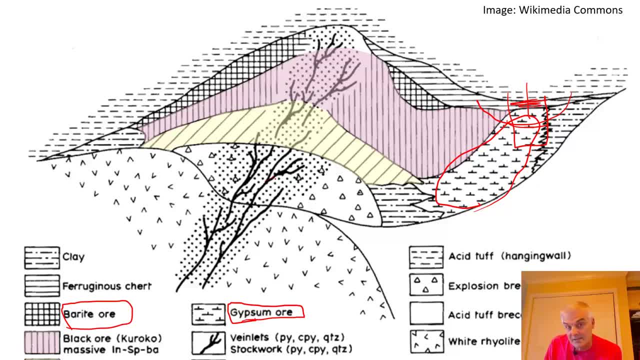 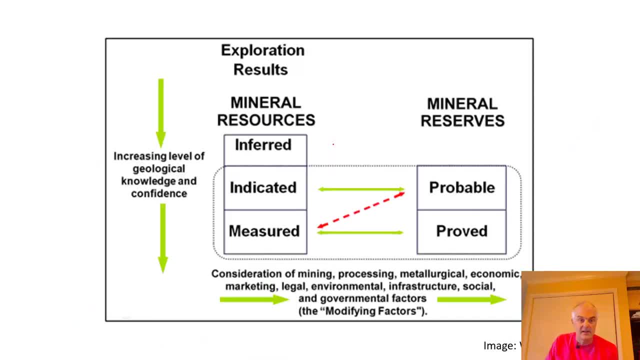 think it through, how you're going to mine it. there's really two kinds: uh, top or underground. right, you go from the top a surface mine, or you dig and like do tunnels and stuff like that. you've probably seen that in movies and stuff like that- and then once you've discovered the ores, last, 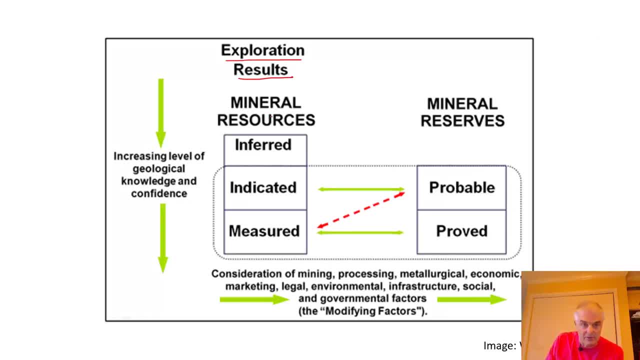 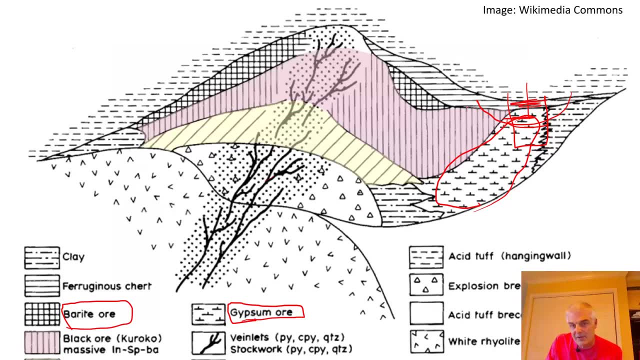 picture here is: you can have what they call the results, right. so there is inferred, so inferred. if you go back here, you actually may not know where all this stuff is. maybe all you know is you've dug down this deep and then you're going to have to. 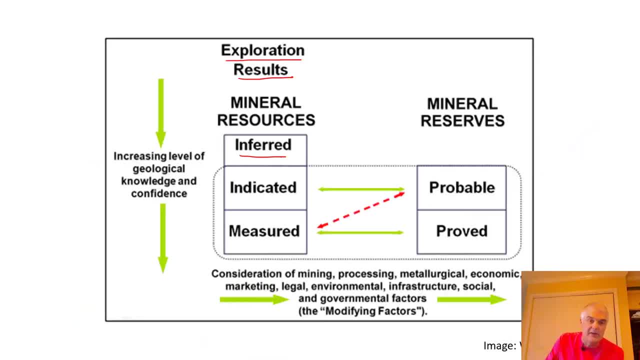 like drill a sample and again all these cost money and then what you've got? some mineral resources. there's much indicated, measured, and then there's also probable. so maybe in this map, maybe they now know this is exactly how much there is, but maybe they only know this depth right here and so they 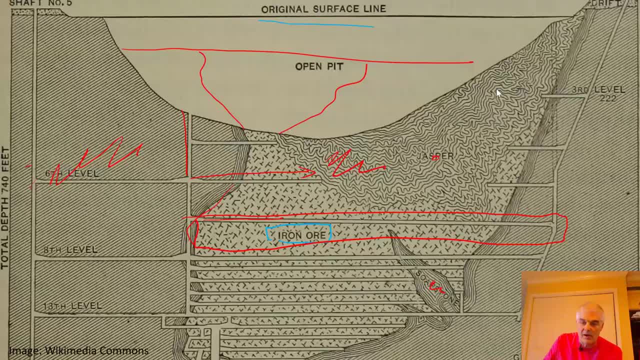 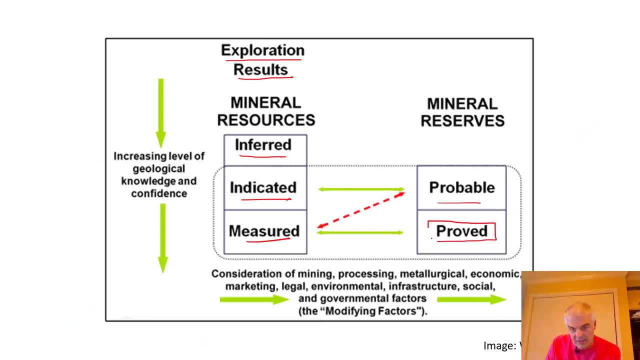 think: well, we think below this. they might be somewhere, so they have these. we call these probable resources that we've gotten and then there's proven now proven. so what a geologist is looking for? this is an exploration geologist's proven resources so they can go at it and get at the valuable minerals and